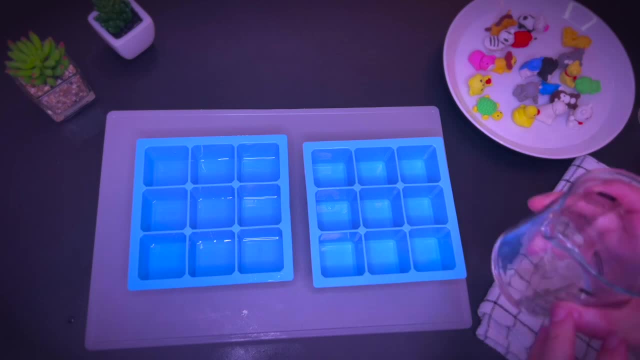 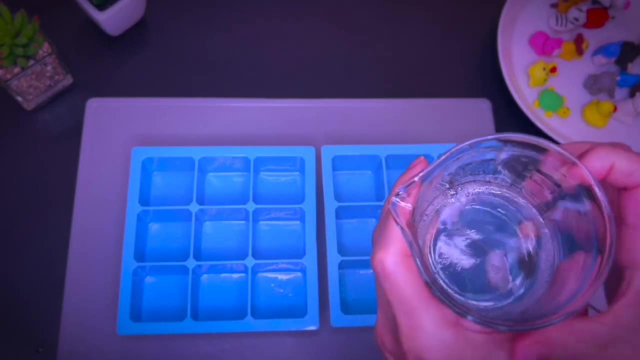 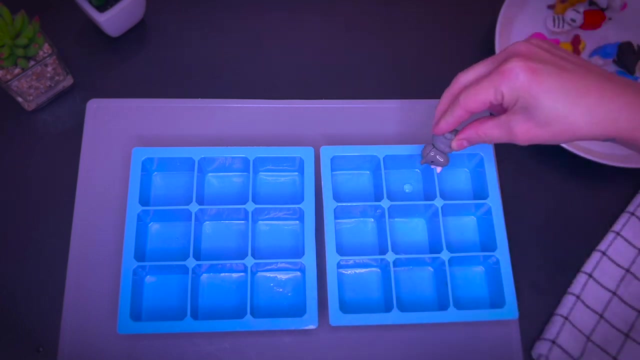 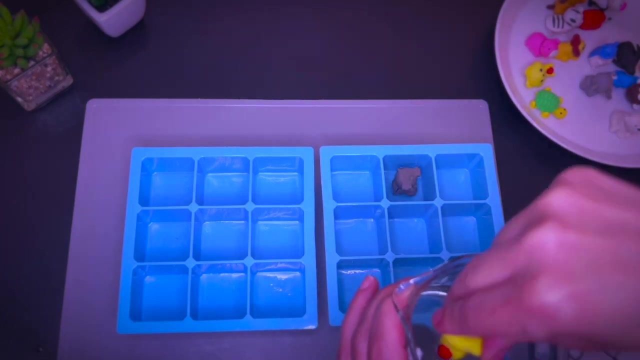 minutes. i grab one of the toys and dip it into the melt and pour and then attempt to glue it onto the thin layer. if that makes sense, you might need to hold it still for a moment until you feel that the soaps or the two elements stick together. 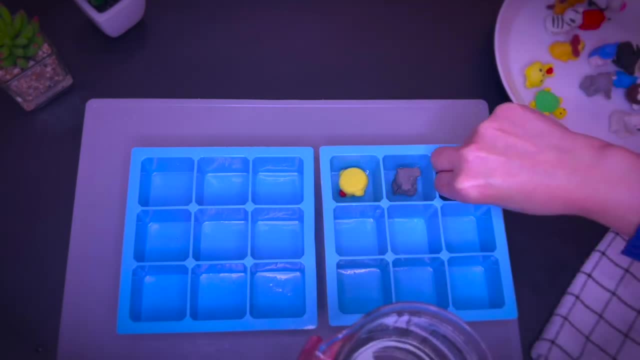 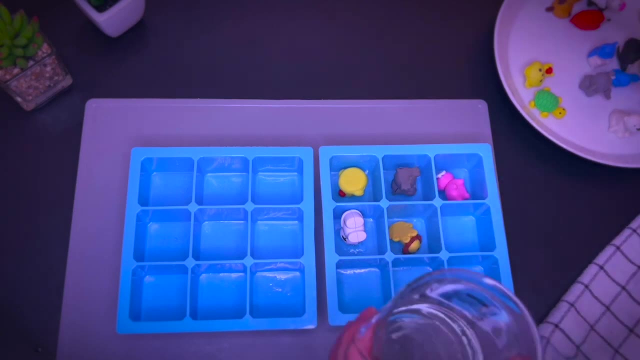 now i'm going to repeat this for every single cavity here you can see that the toy is upside down because the top of this mold has a diamond shape cut that you will see in just a moment. so in this case it looks better this way around you. 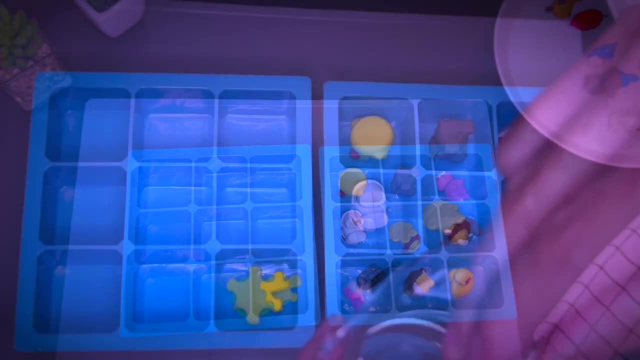 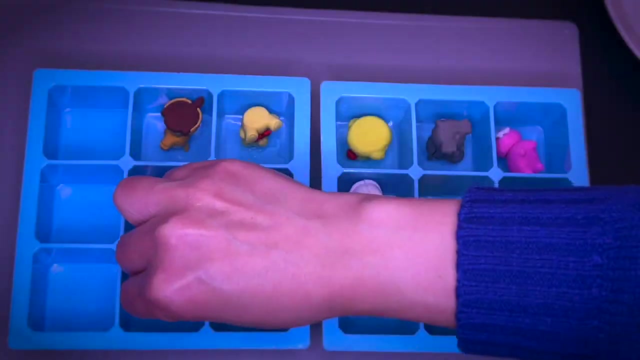 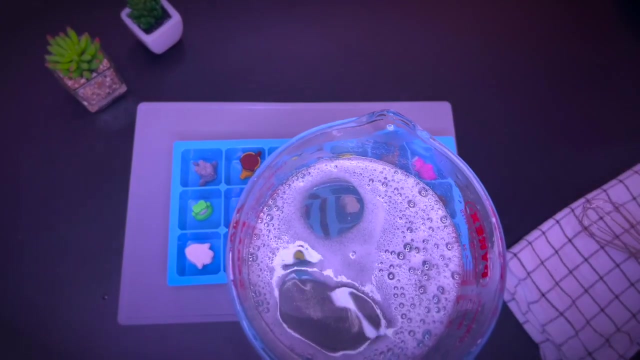 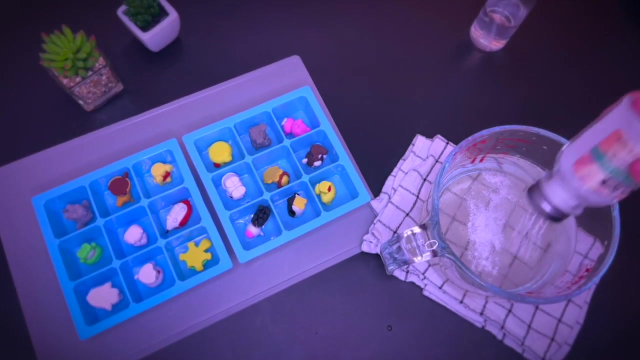 could also do it right side up, and it's actually easier for the animals to stand on their feet. now it's time to color our melt and pour, and the trick here is actually not to color it, or just to color it very, very slightly. try to make it as transparent as possible, so the toys remain. 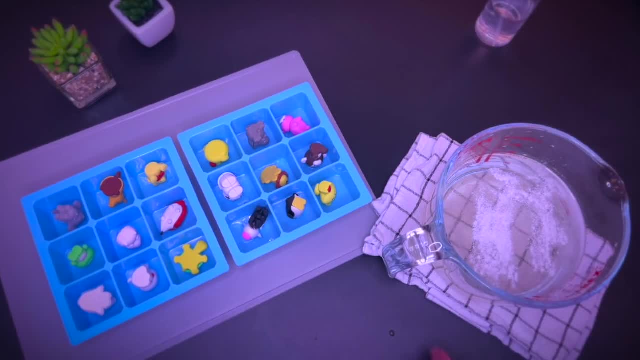 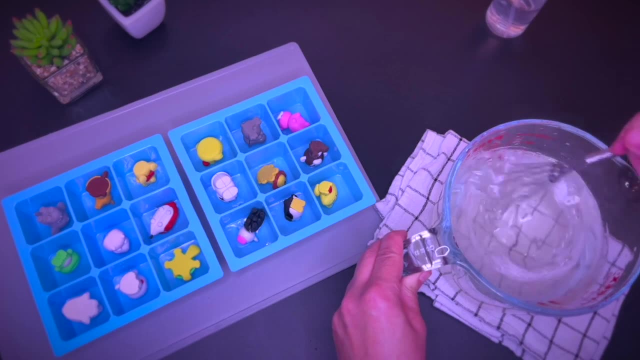 visible. i'm using a biodegradable glitter just to give it a little sparkle. i like to use a whisk to incorporate color with melt and pour. now i'm going to add a little bit of color to the top of the toy and i'm going to add a little bit of color to the top of the toy. i'm going to add a little bit of color to the top of the toy. 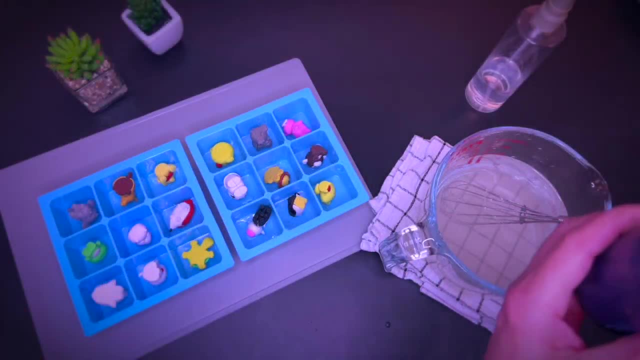 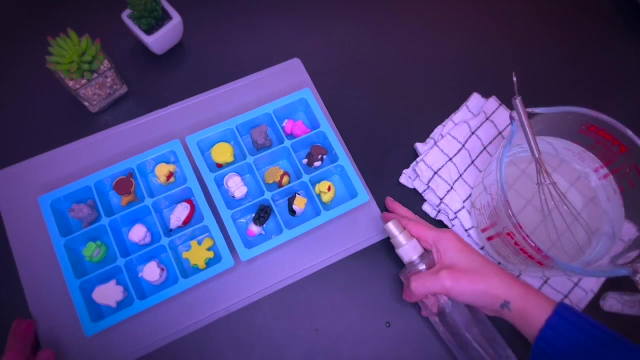 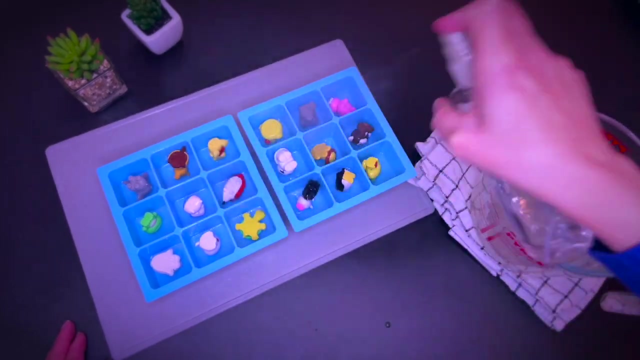 i will also add a fragrance oil. best is to choose one that has a light color to it, so you can keep the soap as transparent as possible. let's give the mold a good spritz with rubbing alcohol that actually acts like a glue to ensure that the soap sticks to the toys well. 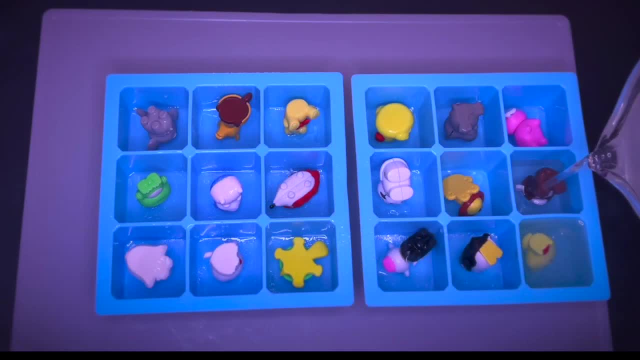 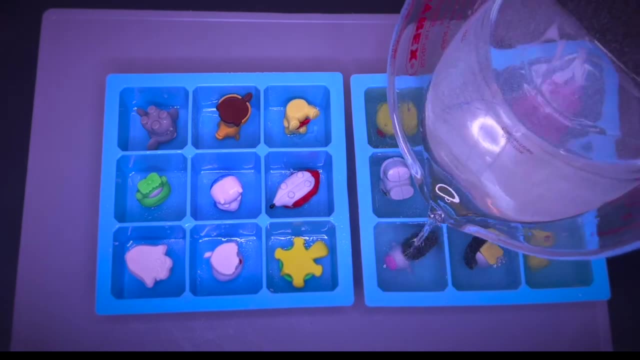 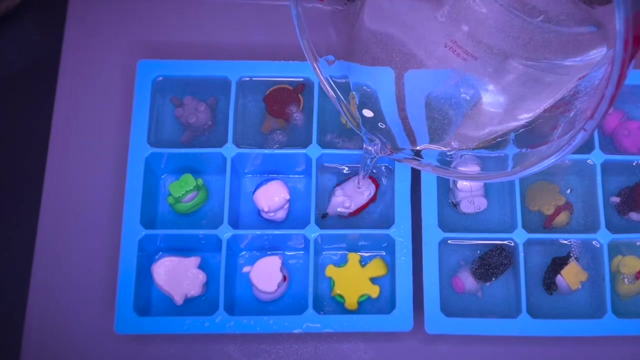 and then i just fill the cavity to the top. by the way, these pyrex jugs are amazing. for a good and smooth pour, definitely worth investing. the only thing left is to wait for one hour or two before unmolding. don't add it to the fridge.